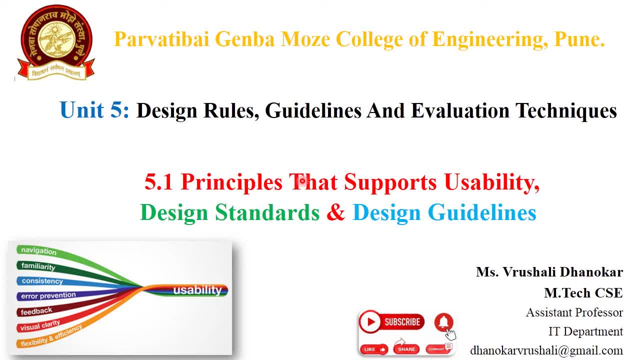 Now, from this video, we will start our next unit, that is, Unit 5.. Unit 5, Design Rules, Guidelines and Evaluation Technique, And the first topic in this unit is Principles. that Supports Usability, Design Standards and Design Guidelines. 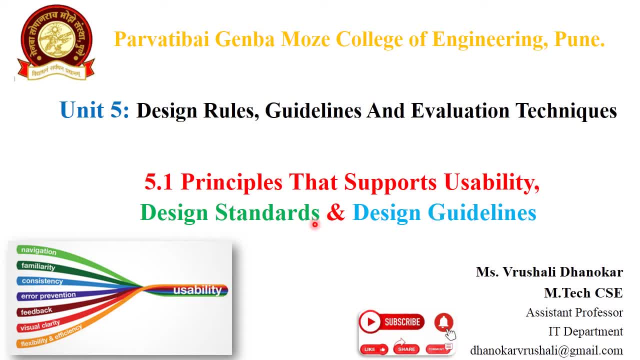 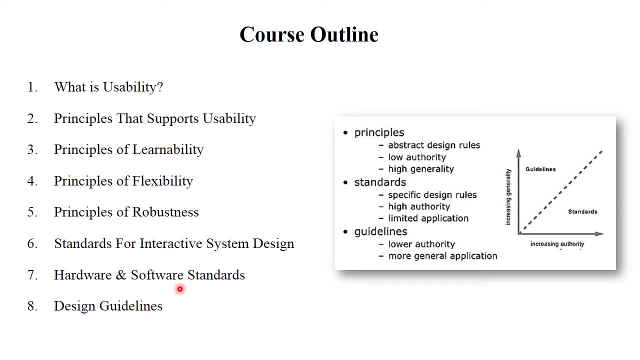 So let's see how exactly these design principles will work Next. Following points are covered in this video, which includes what is usability principles? that supports usability, principles of learnability, principles of flexibility, principles of robustness and also some standards of interactive system design. 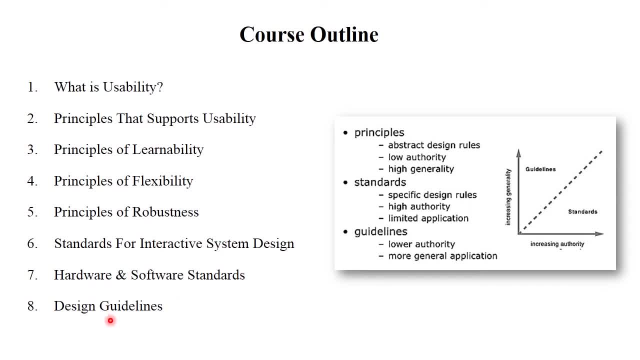 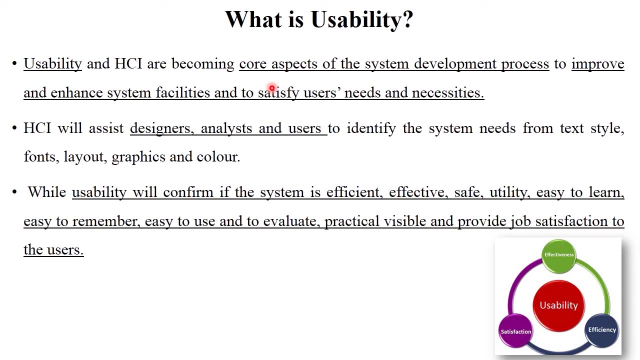 which includes hardware and software standards And, last, design guidelines. So let's see one by one. The first topic is: what is usability? Next, Okay, So we all are familiar with design models and also usability. So let's see what is usability techniques, because we learn all those points in my last videos. 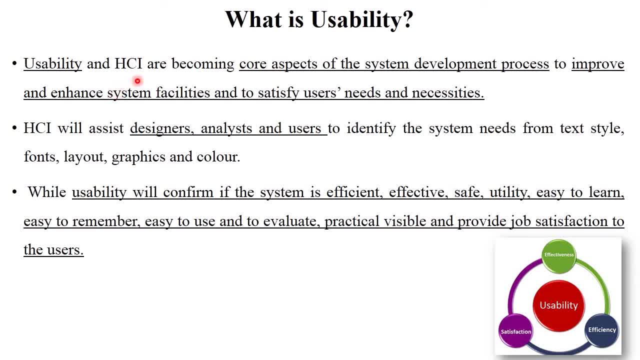 So what is usability? Usability and human-computer interaction are becoming core aspects of system development process. It improves and enhance system facilities and to satisfy users' needs and necessities. HCI will assist designers, analysts and users to identify the system needs from textiles. 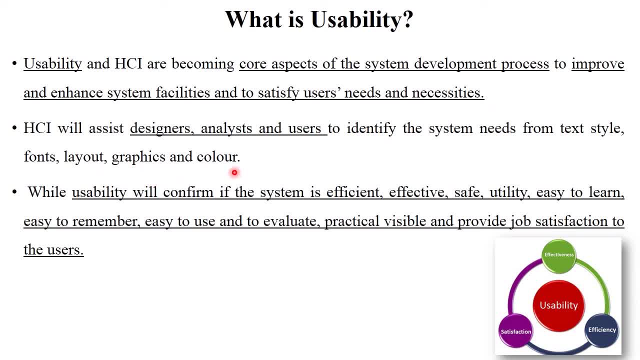 fonts, layouts, graphics and colors, etc. So usability simply means to satisfy the users' needs and necessities throughout software development process. The particular app will be easy to learn and easy to use. So while usability, it will confirm if the system is efficient, effective, safe utility, easy to learn, easy to remember. 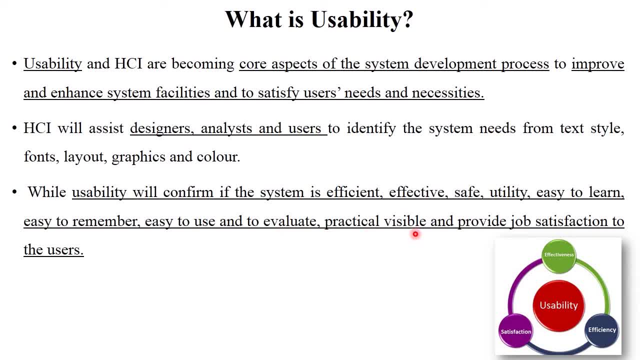 easy to use and easy to use. Easy to use and to evaluate the practical, visible and also provide a job satisfaction to the user. So this is the concept of usability. Usability simply means satisfaction, effectiveness and efficiency in your applications. 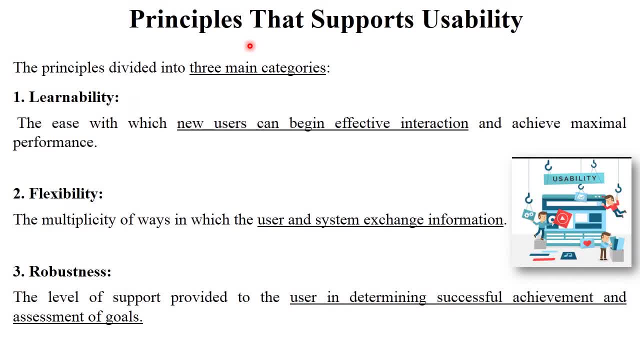 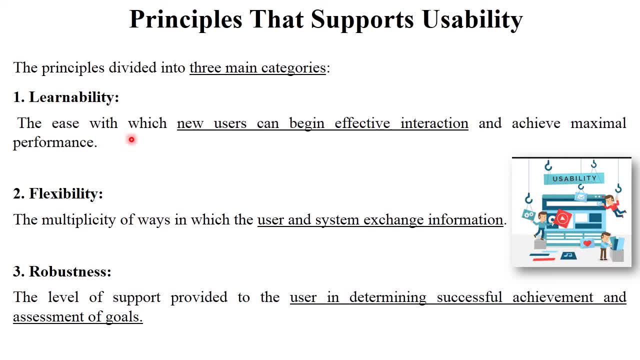 So what is mean by learnability? The learnability means the new user can begin effective interaction and achieve maximal performance. Means each and every users use the particular application as per their requirements. Right. The next: flexibility. Flexibility means the multiplicity of ways in which user and system exchange the information. 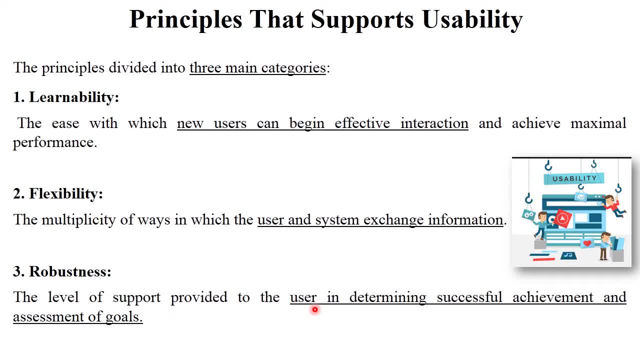 And robustness means the level of supports provided to the user, provided to the user in determining successful achievement and assessment of goals. so these are the principles: learnability means easy to learn to new users, flexibility means easily exchange information from the user and the system, and robustness means to achieve successful goals. 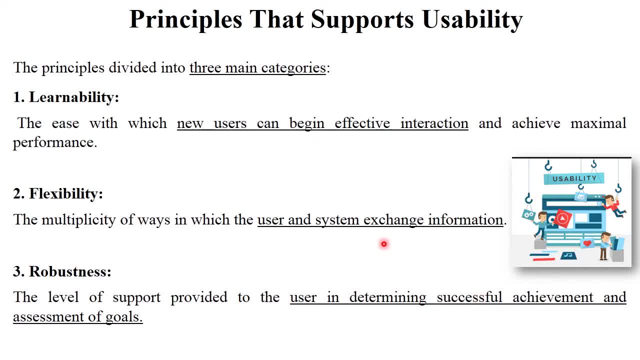 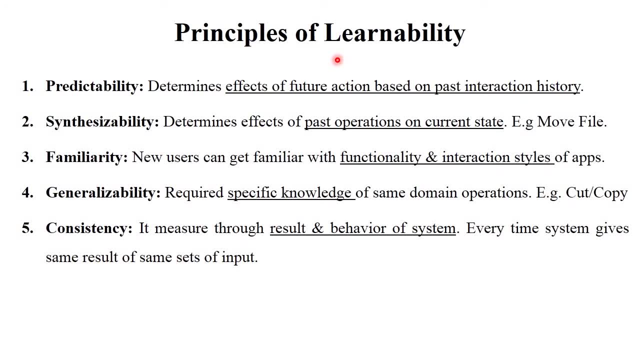 and the requirements clear. so these are the main principles of usability. next, now, the first principle is learnability. again, the learnability principles can be divided into these five principles. the first one is predictability. predictability determines effects of future action based on past interaction history, while develop a particular product. 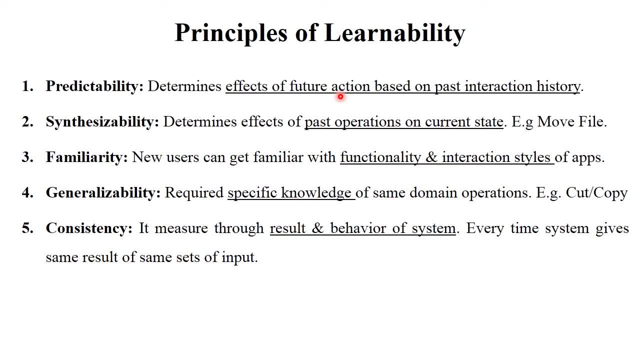 your past action will be effect on the future action. right. the next synthesizer: predictability. it determines effects of past operations on the current state. for example, move file. you should move a file from one folder to another folder, right? so past operation is depends on the current state. next, familiarity: new users can get familiar with the functionality. 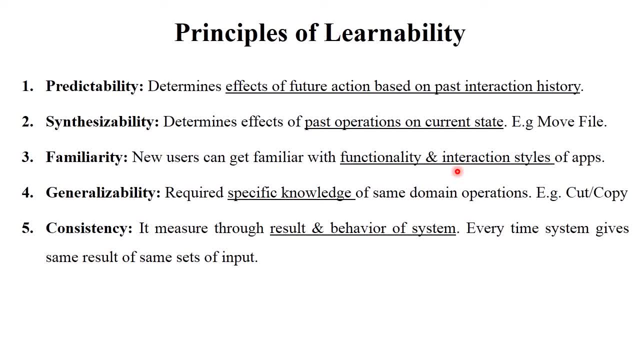 interaction styles- again new features in that particular application: generalizability. it required a specific knowledge of same domain operations. for example, we all are familiar with Microsoft word right, so cut copy paste are the familiar operation, so each and every one know that. how exactly cut copy paste? 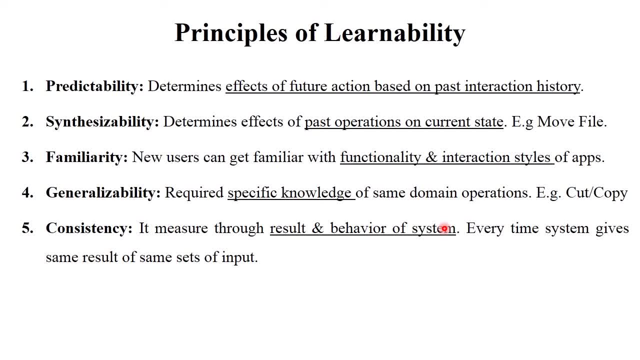 operations will be work and their shortcut keys also. so these are the specific knowledge includes in generalizability. next, consistency: consistency to measure the result and behavior of system every time system gives same result of same set of input. for example, if you should provide two plus two, so system always get the result. that is, four means same set of input, same result provided by the system. so this is called as consistency clear. so these are the principles of learnability. next, 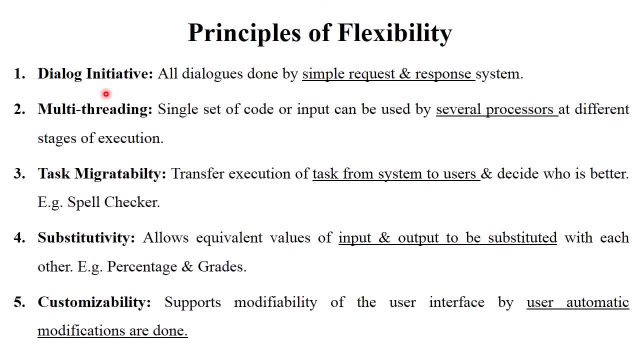 Now the second principle is flexibility. and these are the sub principles of flexibility. First, dialogue initiative. Dialogue initiative means all dialogues are done by simple request and response system. You should request a particular data to the system and system generate the output right. So simple request and response between user and the system. This is called as dialogue initiative. 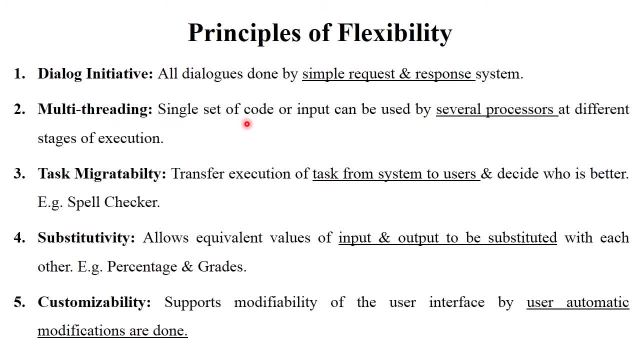 Next, multi-threading. Multi-threading means single set of code or the input can be used by the several processors at different stage of execution. right Next, task migrate ability. It transfer the execution of task from system to users and decide who is better, For example, spell checker. In Microsoft word or in any other document, If spelling get wrong, it automatically change or convert into the correct spelling. 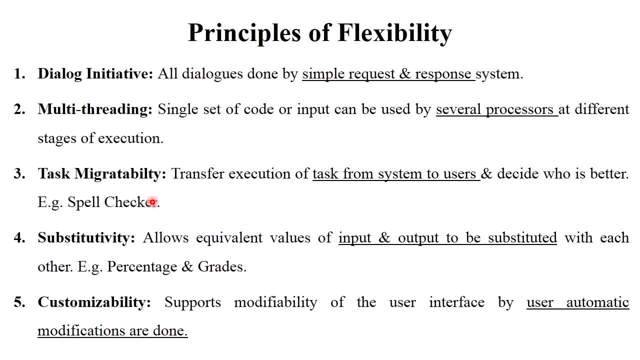 Right So spell checker. Spell checker means you should decide whether the system is better or user is better, Right, So this concept is called as task migrate ability. Next, substitutivity: It allows equivalent value of input and output to be substituted with each other, For example in some Microsoft Excel or Microsoft word or any other documents. 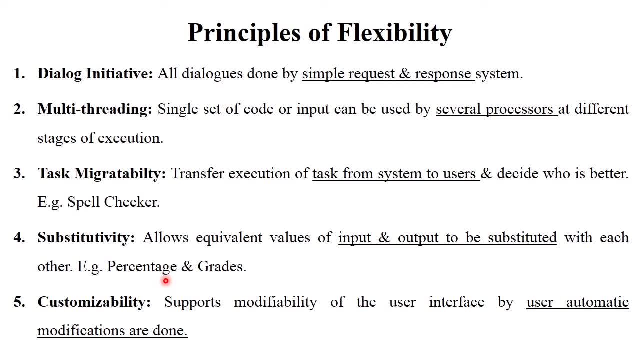 Some data will be given in percentage format, Or some data will be given in grades format, Right. For example, if the percentage more than 80. 80%, So grade will be A. Suppose, more than 60% of grade will be B, So this is called as substitutivity. 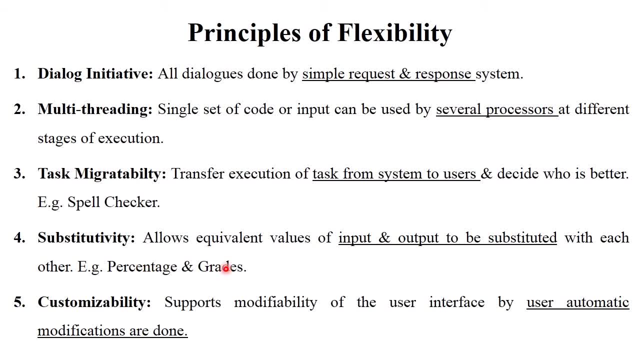 This percentage and grades will be similar. Right. Next customizability: It supports modifiability of the user interface By user. automatic modifications are done. Next customizability: It supports modifiability of the user interface By user. automatic modifications are done. You should customize your app. 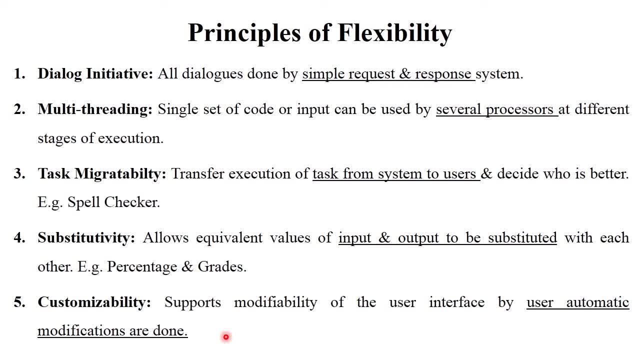 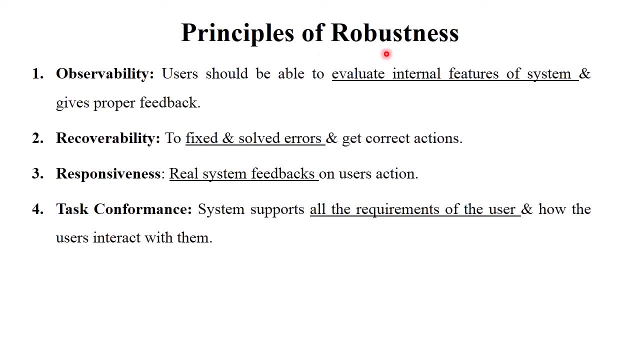 Also, you should use same features and app in one folder, Right? So this is called as customizability. It also done by the user Clear Next. Now the next and last principle is robustness, And these are the sub principles of the robustness. The first observability: User should be able to evaluate internal features of the system and gives proper feedback. 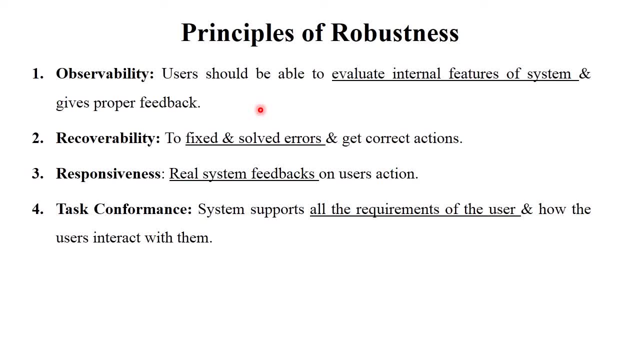 Clear Next. Now, the next and last principle is robustness, And these are the sub principles of the robustness. User should be able to evaluate internal features of the system and give proper feedback. It means that you should analyze each and every feature, For example, the particular media app, for example WhatsApp, So users evaluate the internal feature, like chatting, Then video, audio calls, etc. Right, 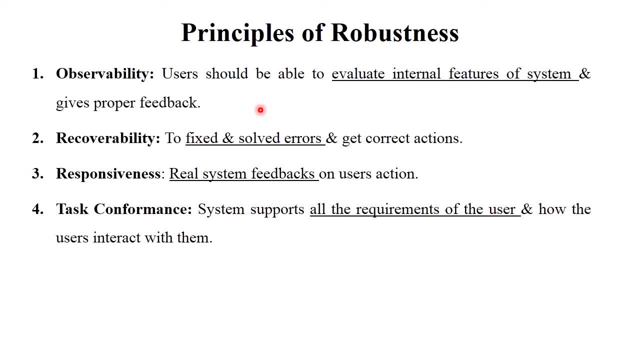 for example, Whatsapp. So users evaluate the internal feature like chatting, Then video audio calls, etc. Right. So user evaluate the internal features of the system and it gives proper feedback to the particular application. For exampleäusr if oule keinelei upcoming feature: Right The next recoverability. moetper victorious apps: Right The next recoverability. It features and solve the. 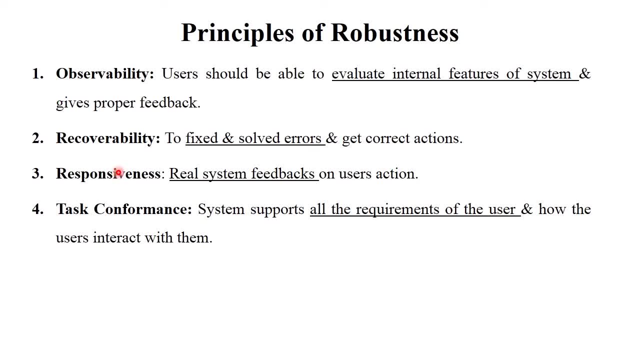 and solve the errors and get correct actions. responsiveness means real system feedback on the user's action, how exactly system work after the deployment. here next task: conformance system supports all the requirements of the user and how the user interact with them. there are different types of applications are developed as per the requirements or as per the field of the user. 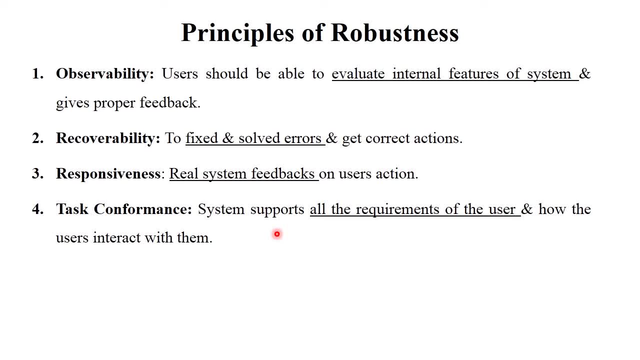 right. so system supports the each and every requirements of the user. that was the main aim or the goal. so this principle is called as task conformance clear. so these all are the principles of the design. you should analyze and evaluate all the principles while development a particular. 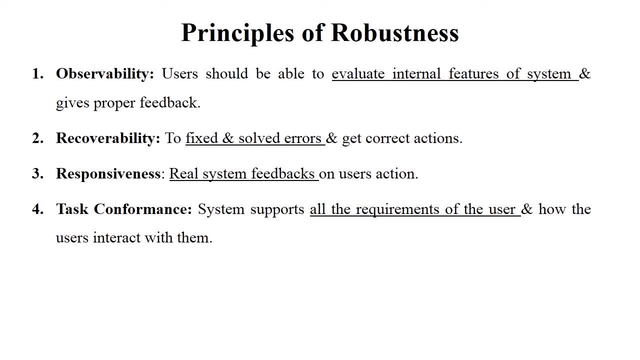 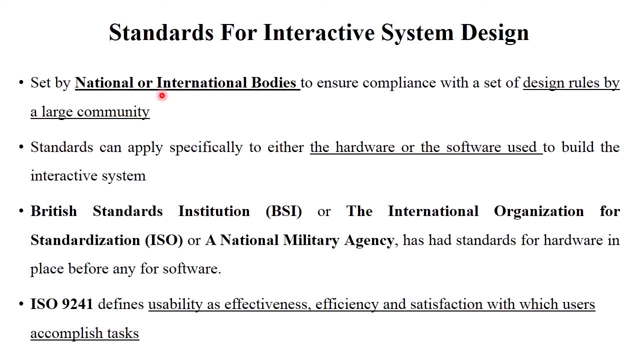 software or particular application. only that your application will be more quality and more quality products will be generated- clear. next, the standards for interactive system design. there are different types of standards set by national or international bodies to ensure compliances with set of design rules by a large. 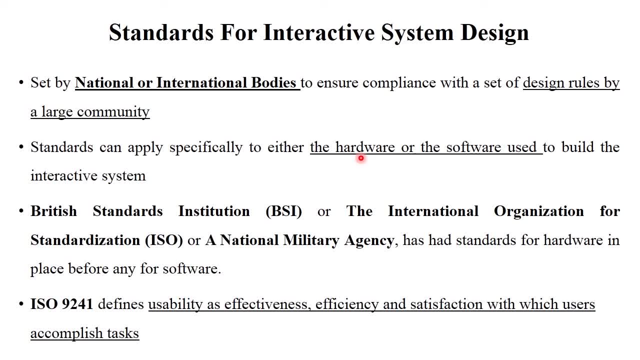 community standards can apply specifically either hardware or software used to build an interactive system. there are some british standard institution which is also called as bsi, or the international organization for standard, iso or national military agency. we know that iso standard. iso standard gives proper standards than hardware and software. purpose with best authority of the particular. 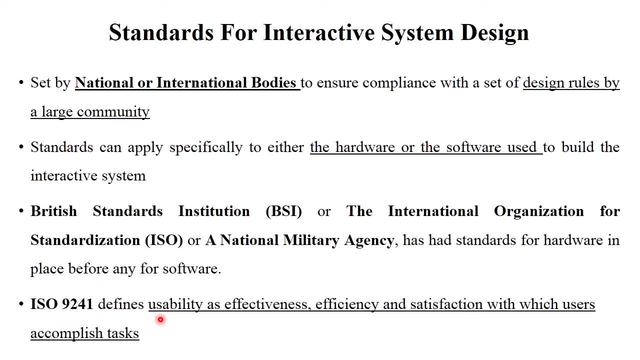 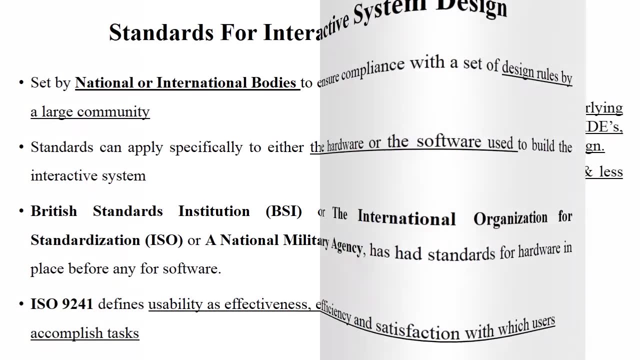 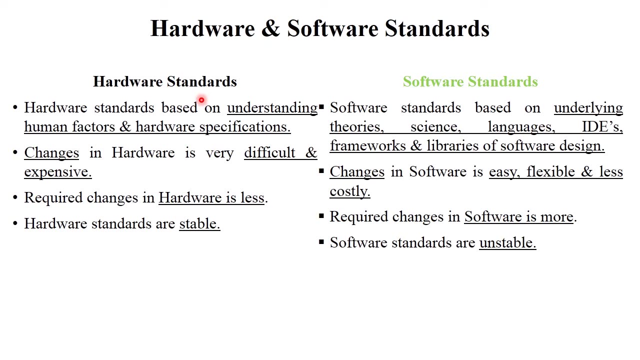 product. the next iso 9241 defines the usability as effectiveness, efficiency and satisfaction with which users accomplish a particular task. so all the principles that will be verified by this iso standard right next. the next one is hardware and software standards. so what is mean by hardware standards and software standards? each and every product will be get through iso standard, that is. 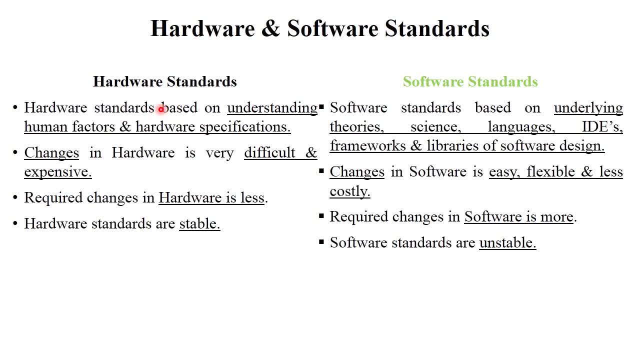 authorized global products. okay, so hardware standards means hardware standard based on understanding human factors and hardware specification. the changes in hardware is very difficult and expensive. also, right, our mobiles. our mobile are developed by different hardware products. so changes in that particular hardware or particular gadgets is very difficult and expensive. the part of that particular hardware product is also 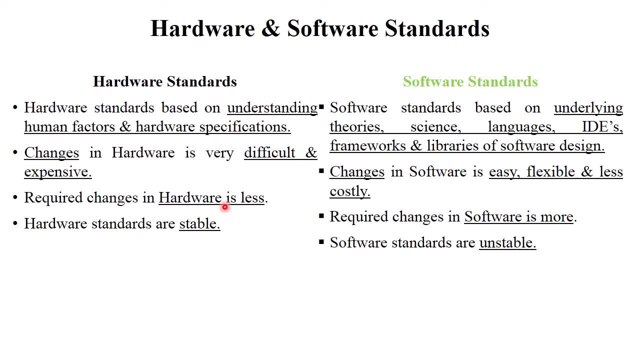 expensive right, so required changes in hardware is less and hardware standards are stable. now what is mean by software standards? software standards based on underlying theories, science, languages, ids, frameworks and libraries of system design is a very difficult and expensive software to develop. it should use different types of frameworks. 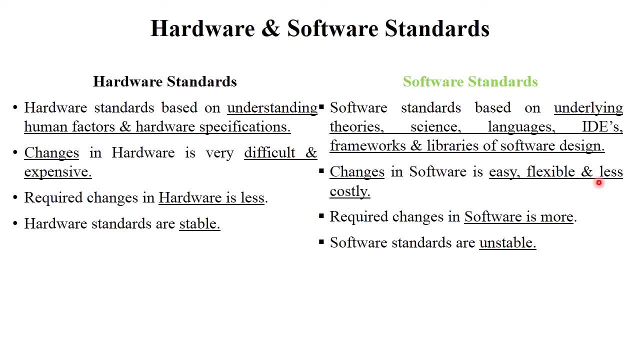 programming languages for develop a particular software. so changes in software is easy, flexible and less costly. there are some alpha, alpha, beta. this kind of versions are developed of particular software. right, so it should. it used a previous features and also add some new features in your applications, right. so required changes in software is more. 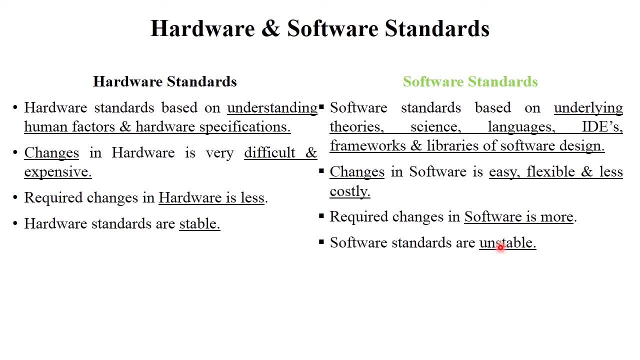 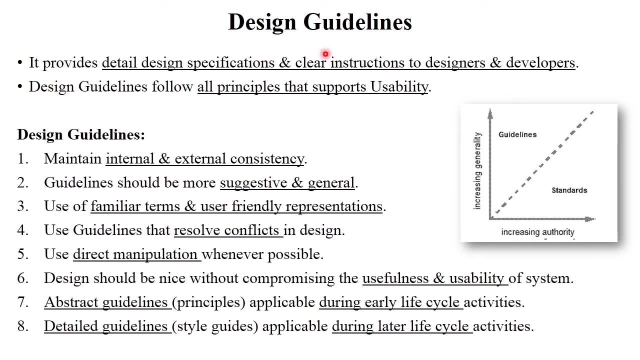 You should add different features or extra features in your applications Clear, So this concept is called as hardware and software standards. Next, The next topic is design guidelines. Design guidelines is one of the most important point, or important guidelines. While design a particular software or particular product, It provides a detailed design specification. 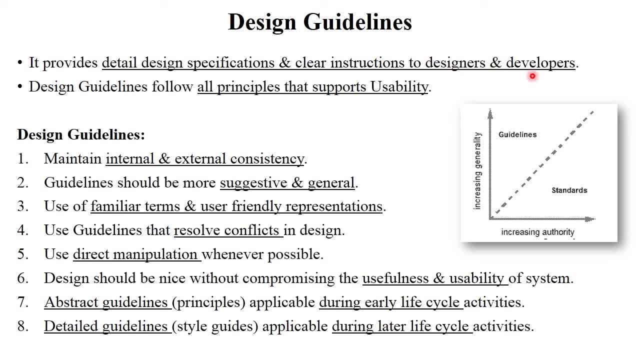 And clear instructions to designers and the developers. It must to follow each and every guidelines and rules for design a product. Design guidelines follow all principles that supports usability Right. So what are the design guidelines? Design guidelines maintain internal and external consistency. Particular app will be developed as per their internal features and also external frameworks. 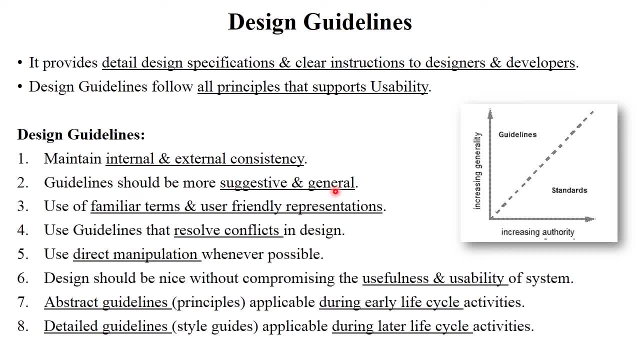 Right. The next guidelines should be more suggestive and general User-Familial terms and user-friendly representation. For example, in Microsoft word there will be option That is, file, new, file, cut, copy paste, edit, etc. So these are all our familiar terms. 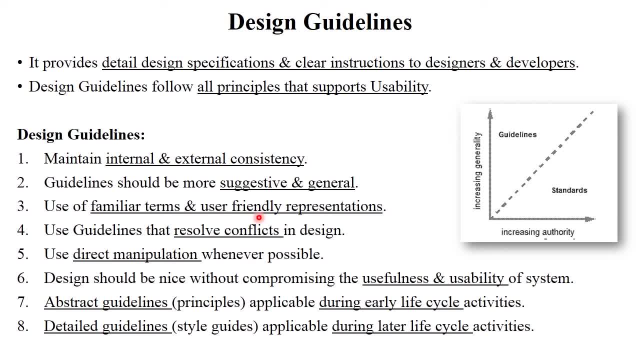 Each and every person, whether it is technical and non-technical, use this product. So use guidelines that resolve conflicts in design. Use direct guidelines that resolve conflicts in design. Use direct guidelines that resolve conflicts in design. Use direct manipulation whenever possible. Design should be nice without compromising the usefulness and usability of system. 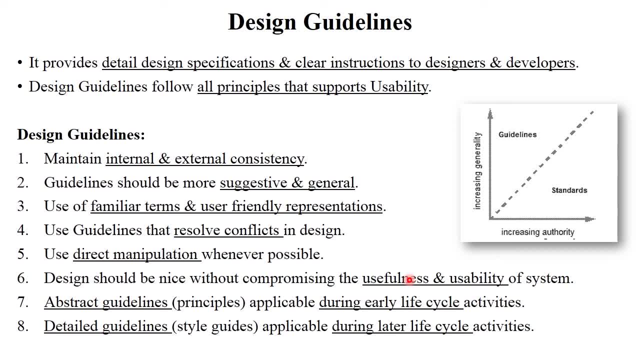 You should maintain the usability and usefulness of particular product. Don't be compromise in that design rules. The next, abstract guidelines. Abstract guidelines means principles- All the design principles Which will be applicable during early life cycle activities- And detailed guidelines. Detailed guidelines means style guidelines, How exactly your product will be look in future.